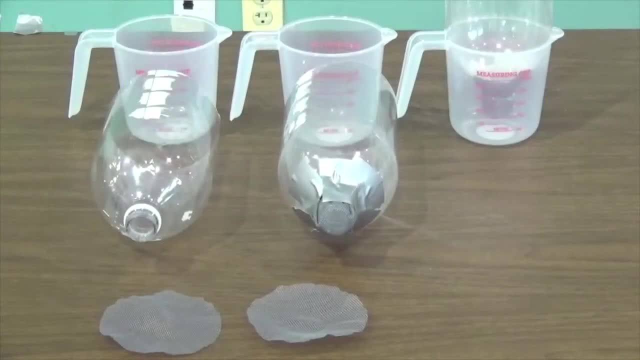 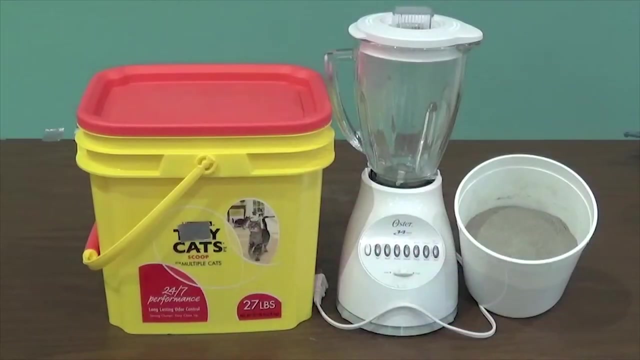 materials you're going to need to get started. You'll need three 2-liter soda bottles with the base cut off, six pieces of fine window screen cut into circles and three measuring cups Water with food coloring. You'll need three cups of clay kitty litter ground up in a blender. 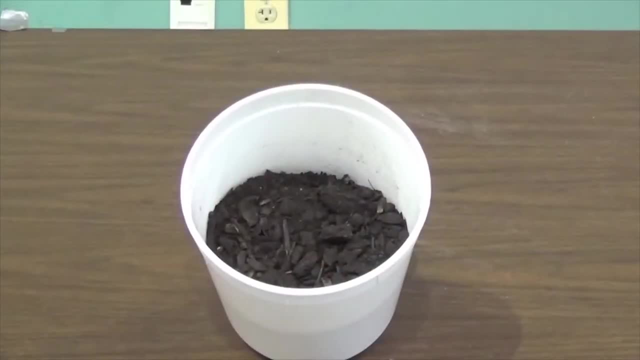 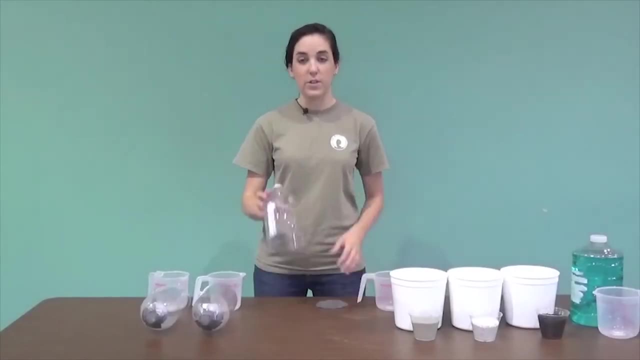 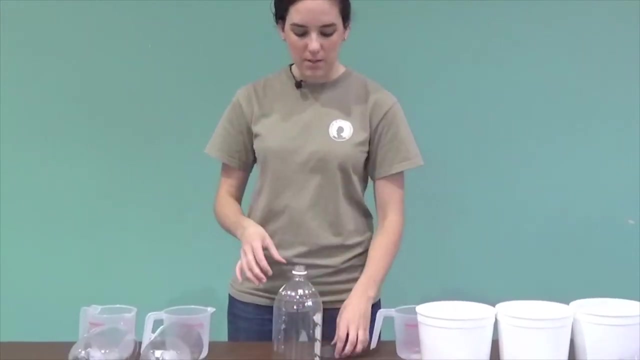 three stopwatches, three cups of potting soil or local soil, four or five cups of sand. So your first step is going to be to cut the bottoms off of your soda cans- So I already have this one cut here- And your second step is going to be to take your window screen. you'll have two pieces. 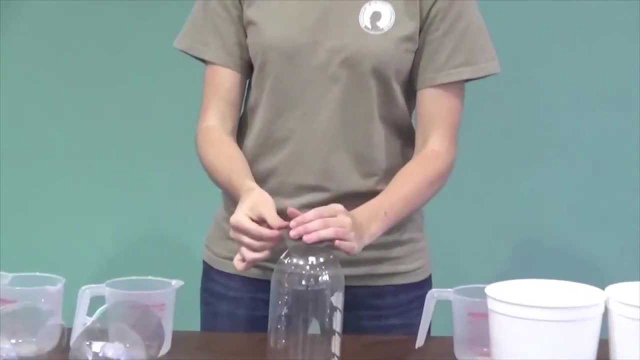 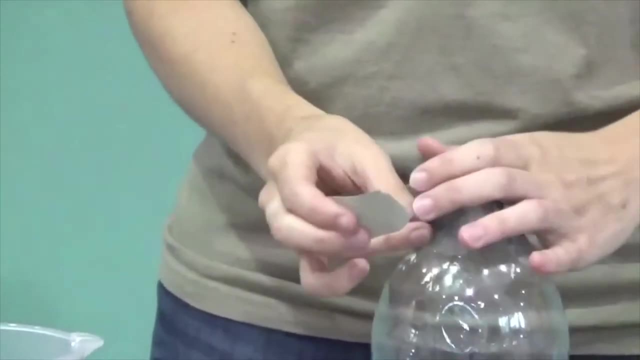 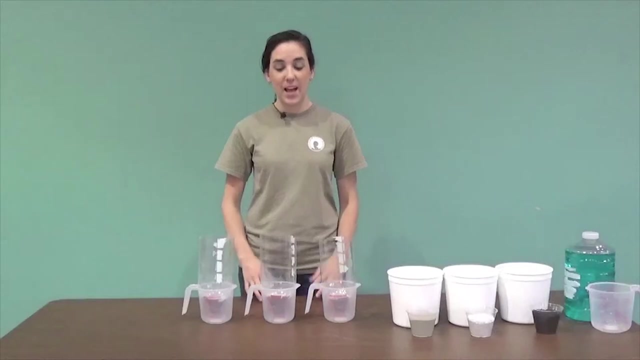 put them on top of each other and attach them to the top of the bottle like this. You'll use some tape to keep that in place. So once these are all taped up, they're going to look like this. So they're taped all the way around here. After you're done taping the screen onto the bottles. 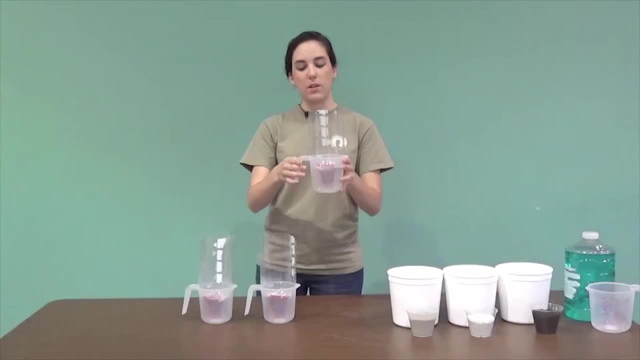 you're going to want to place each of them into the measuring cup. One thing you want to do is make sure that the bottom of your soda bottle isn't touching the bottom of your measuring cup. here, The next thing we're going to do is add a third of a cup of sand to each one of these. 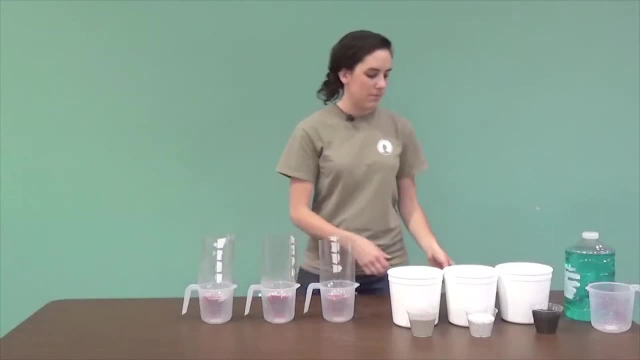 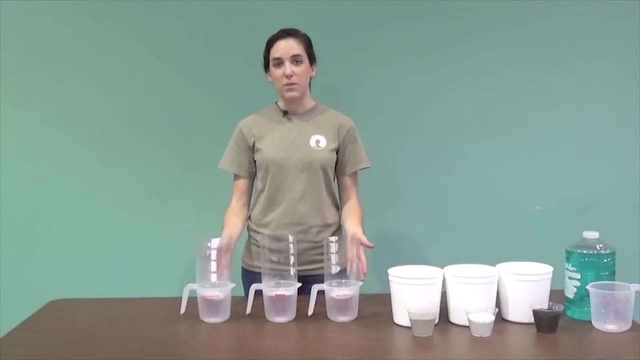 bottles to keep the screen at the bottom clear. After you're done filling each of them with a third of a cup of sand, you're going to want to add three cups of additional material. So in the first one here we're going to add three cups of the potting soil, And then we're going to add 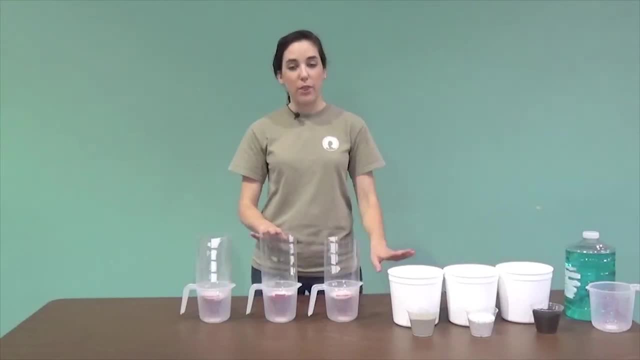 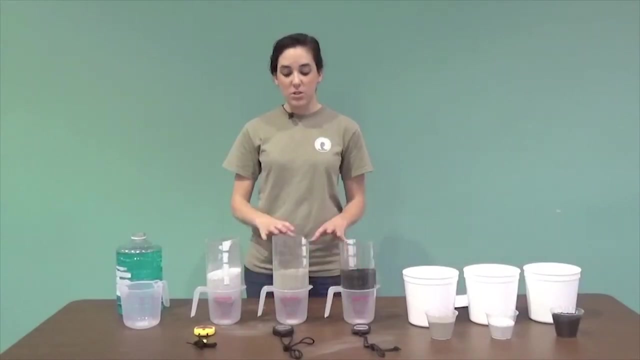 the potting soil or your local soil. And the second one: we'll add three cups of the ground up clay, kitty litter, And then the third one: we'll add an additional three cups of sand. So now that you've added three cups of the different soil types to each of your containers, 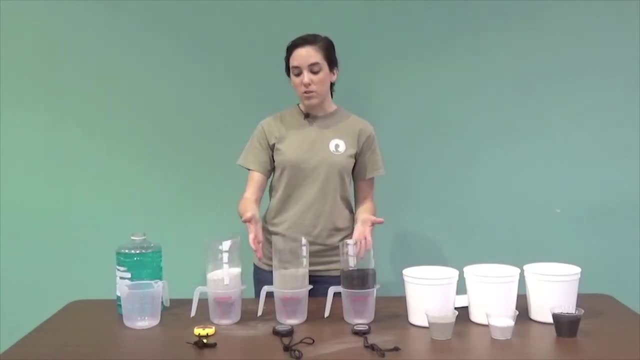 you're ready to run the experiment, So make sure you've taken your stopwatches out And some things you want to discuss with your students before you run. this would be: how fast is the water going to move through each of these soil types? 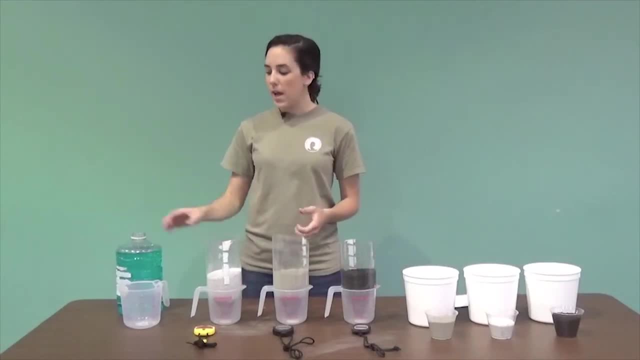 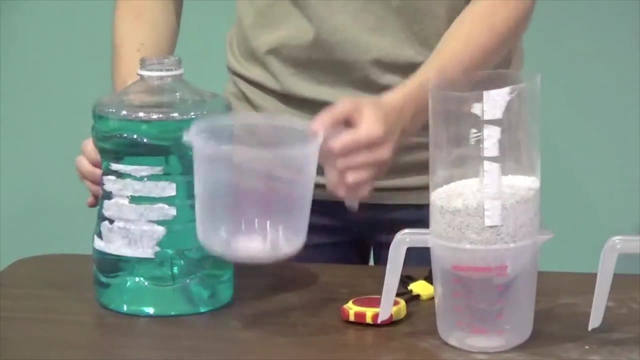 Whether the soil is going to absorb any of the water and how the color of our food coloring water might change from the top to the bottom. So we're going to run the sand first. What you want to do is measure out two cups of water. 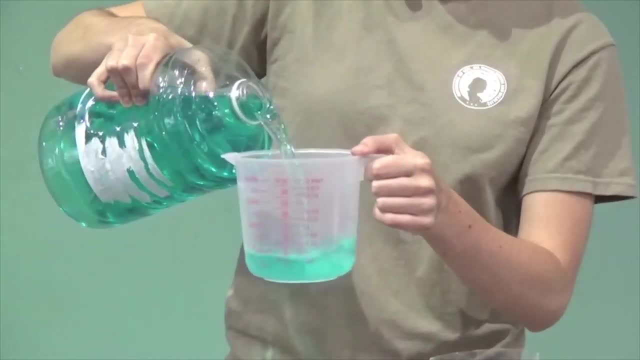 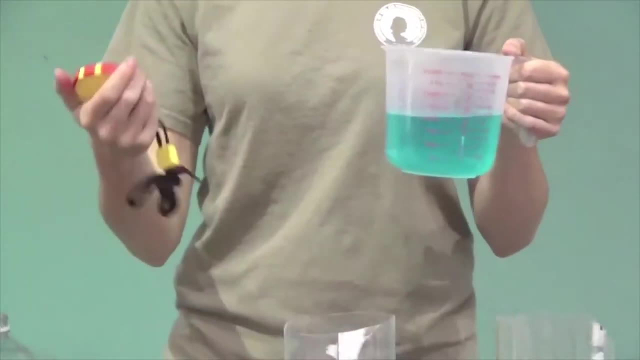 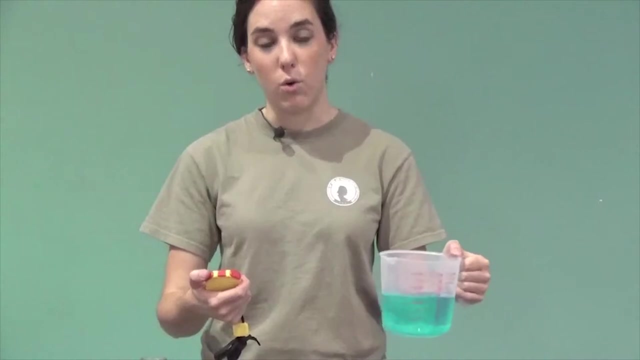 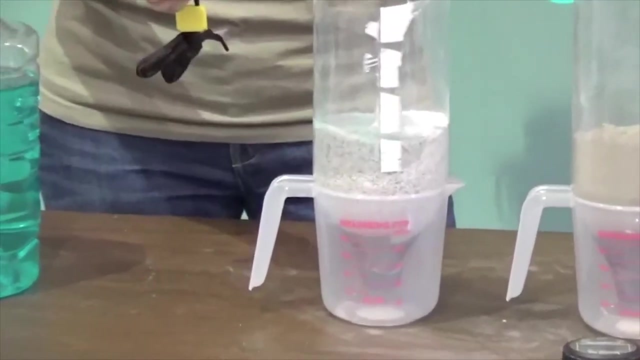 and you want to start your stopwatch right when you start pouring. when you pour the water, make sure that you or your students don't just dump it right in. you want to pour it evenly over the whole container. so we'll start timing when we start pouring and you're going to watch for when. 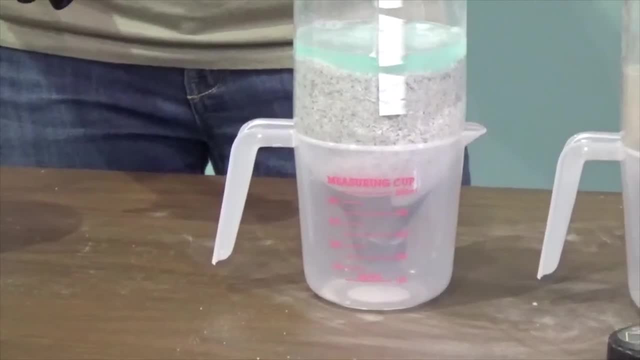 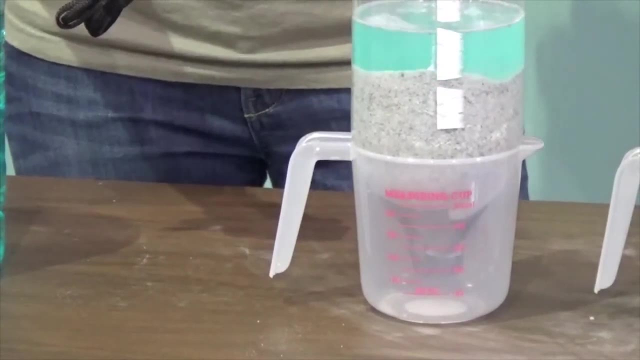 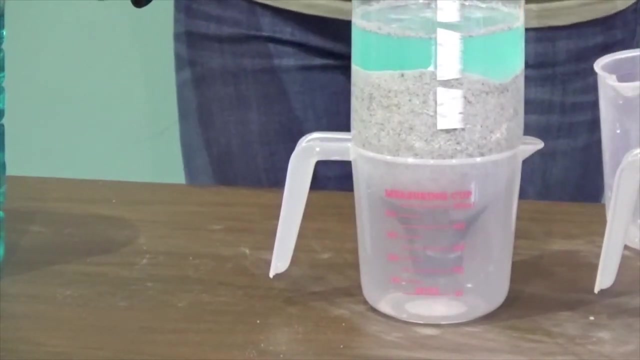 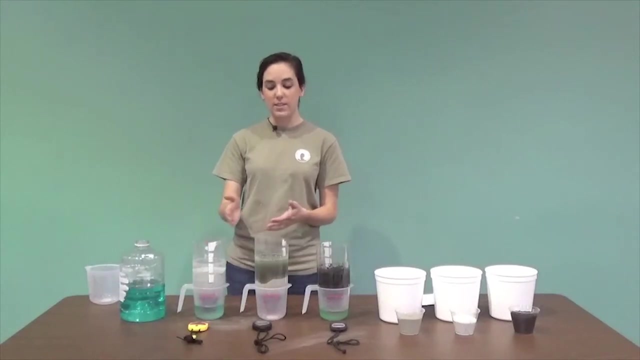 the water starts to come out of the bottom and that's when you'll stop your time. so wait and watch for the first drip to come out, which is at 21.47 seconds for this experiment. so we ran the sand and you saw that come through, and now we put the same amount of water. we put two cups in our 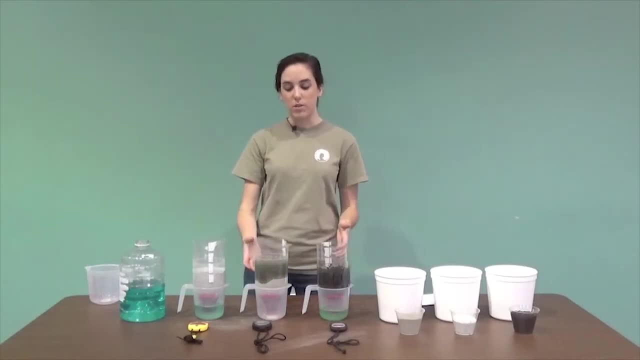 clay soil and we're going to pour that into the container and we're going to pour that into the soil and in our potting soil and let those run as well. so, as you can see, our clay soil here has yet to reach the bottom. we still have some dry clay here and our potting soil went through and 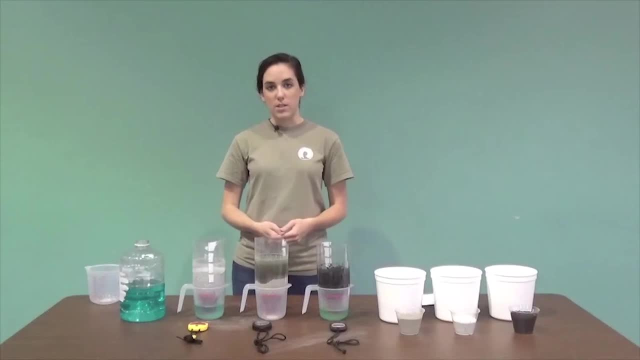 we have some water at the bottom. so there's three things that you're going to want to discuss with your students about this. the first is the timing. so we had stopwatches for each one and we timed them. from the second we started pouring to the second, we saw a drip come at the bottom. for the 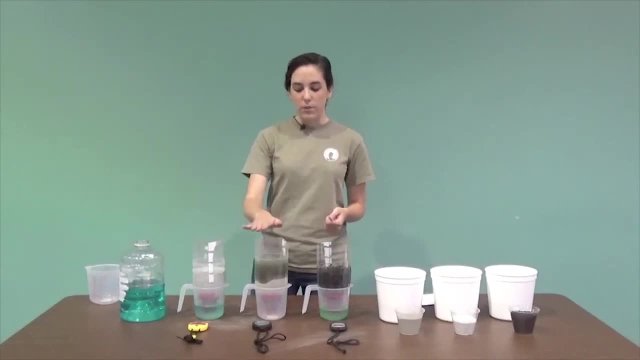 sand that was 21 seconds and for the clay it's still running. for the potting soil it was actually 20 seconds. so the story behind this is talking about poor space within soils. the sand we had was very fine so there was some open air, that poor space in the soil, so it was able to run through. but it did take 21 seconds to do that. the 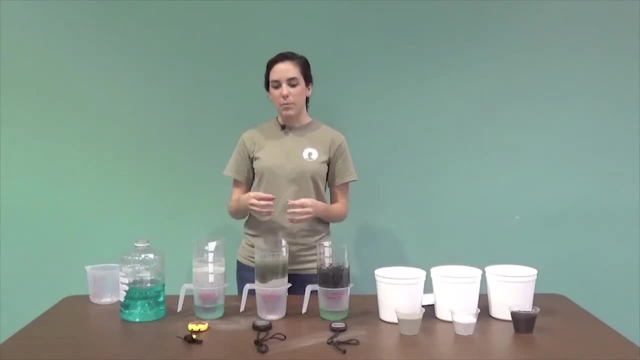 clay has very fine particles, so there's not a lot of pore space, hence why we're still waiting for that to drip through. and the potting soil that we used was very light and fluffy. when we poured the water in, we even had air bubbling up, so there was a lot of pore space in this, hence the 20 seconds that it took to run. 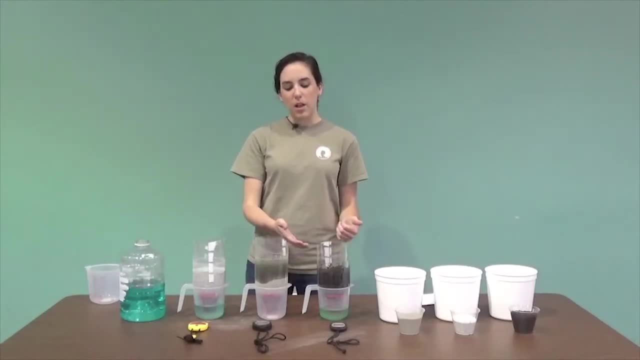 through. if you're going to use a local soil, it's probably going to be a lot longer because, um, that's what's likely to be more dense than this fluffy potting soil that we used, so your results could vary on this one. the other two controls here- the sand and the clay- would usually be pretty.